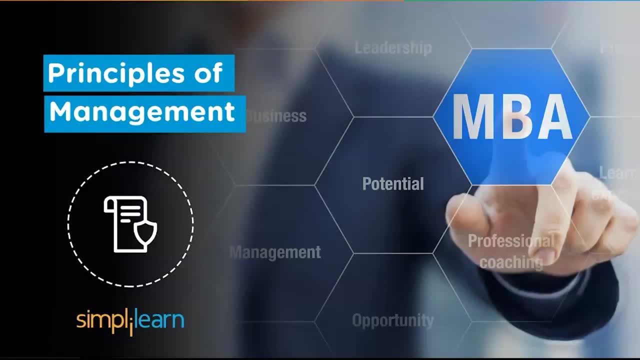 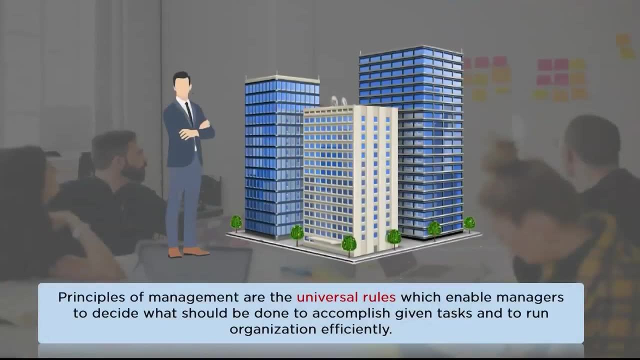 made employees good at their occupation did not necessarily make them good managers. That is why every manager and leadership team should implement rules and regulations to run the organization efficiently, And principles of management are nothing but the universal rules or truths which enable managers to decide what should be done to accomplish given tasks. 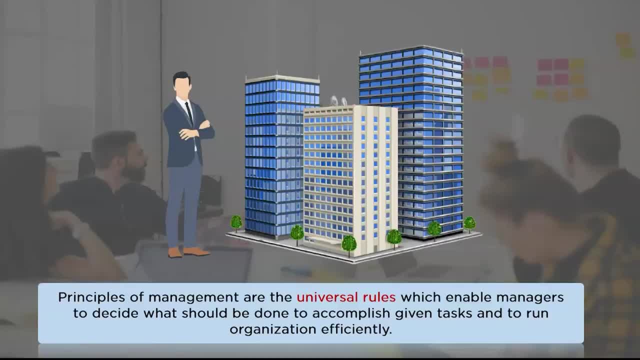 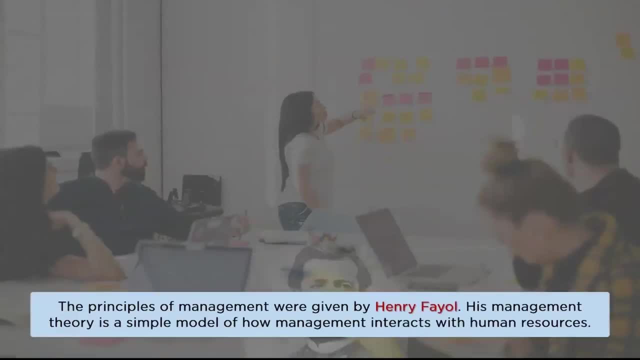 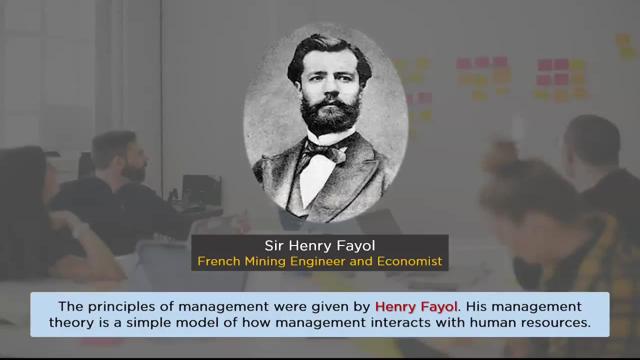 and to handle situations that may arise in management. These principles can be applied to different industries and sizes of enterprises, And all these were given by Sir Henry Fayol. Initially, he started as an engineer and rose through the ranks of the Decazeville mining. 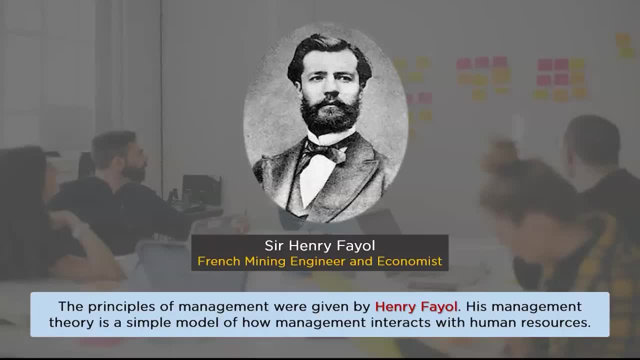 firm in France towards the tail end of the industrial revolution. The faltering company thrived under his leadership. He wrote: When I took the duty for the restoration of Decazeville, I did not rely on my technical supremacy. I rely on my abilities as an organizer and 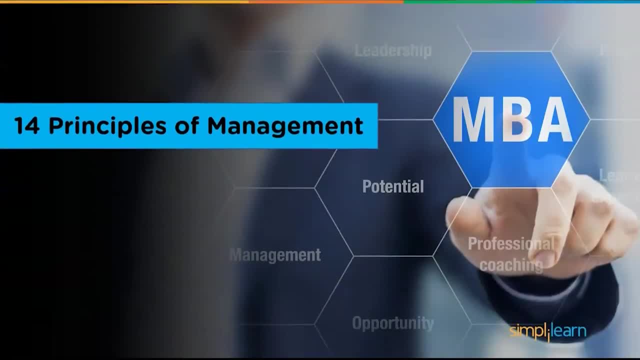 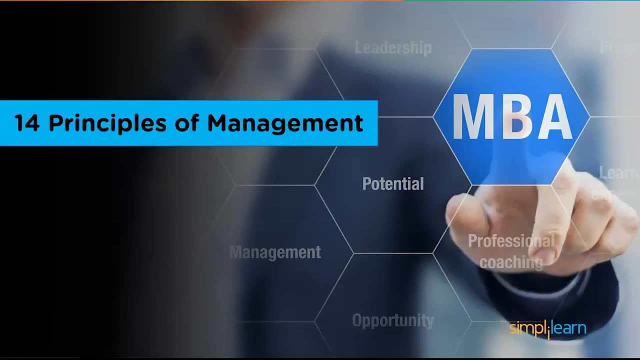 my expertise in dealing with others. So in today's session we'll look at 14 principles of management given by Sir Henry Fayol in his book General and Industrial Management. But before we begin, make sure to subscribe to our YouTube channel and hit the bell icon. 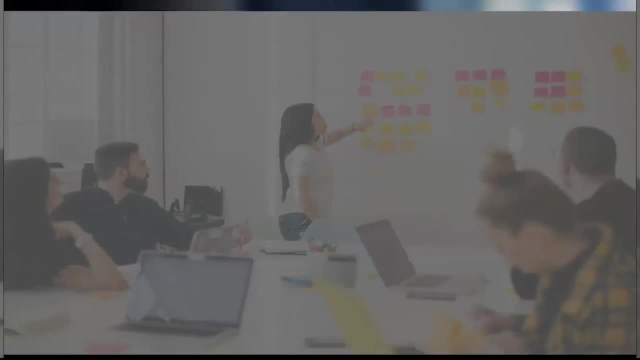 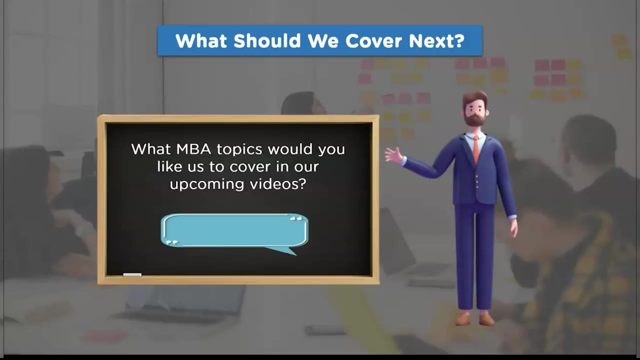 to never miss an update from Simply Learn. Also, if you have doubts about any MBA topics you want us to address, then please let us know about it in the comment section below, and we'll surely create an exciting video about it in the next few days. So guys make. 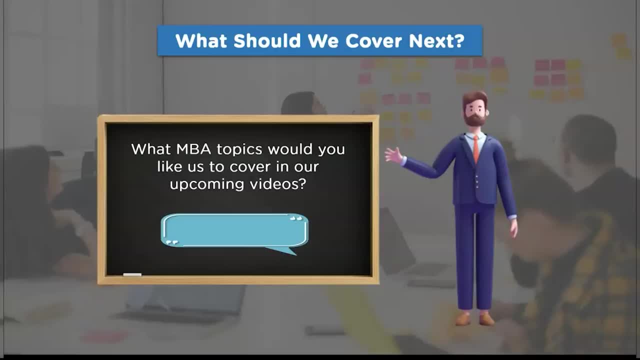 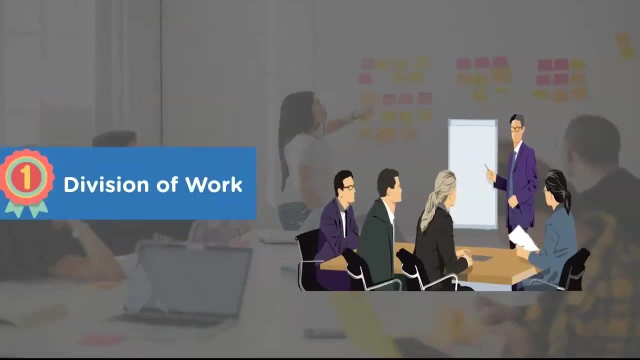 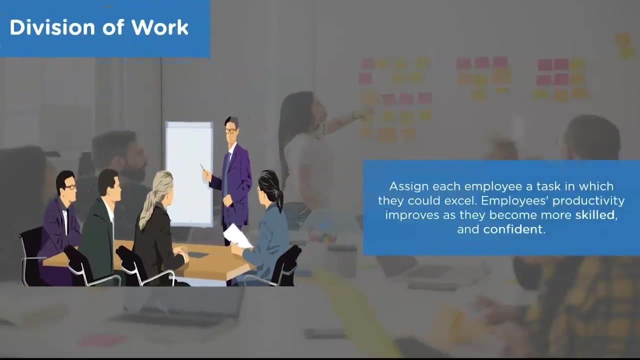 sure you post a comment with MBA topics you'd like us to cover in upcoming videos. Now, coming back to the principles of management, the first principle we have is division of work. This principle states that, as far as possible, the entire task should be divided. 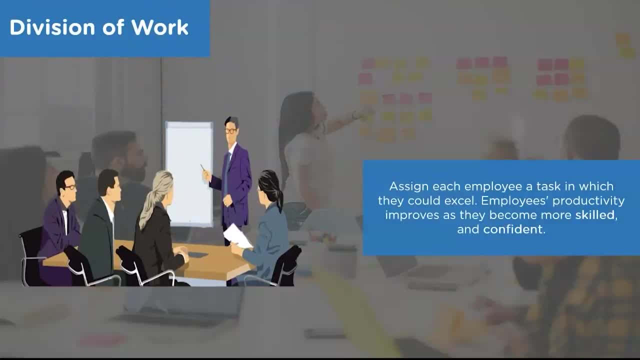 into segments, And each individual should be assigned only one part of the work based on his aptitude and preference, rather than assigning the entire work to one person. When a person does the same task over and over again, he becomes an expert in that particular aspect of the. 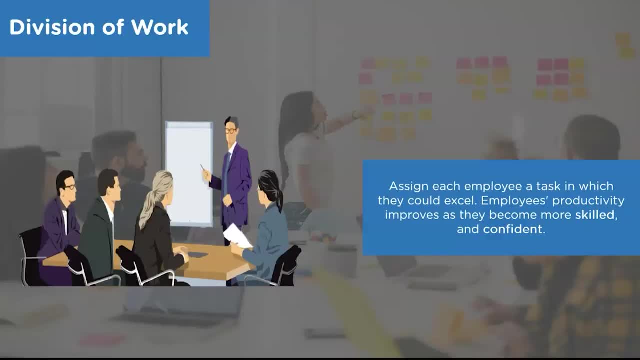 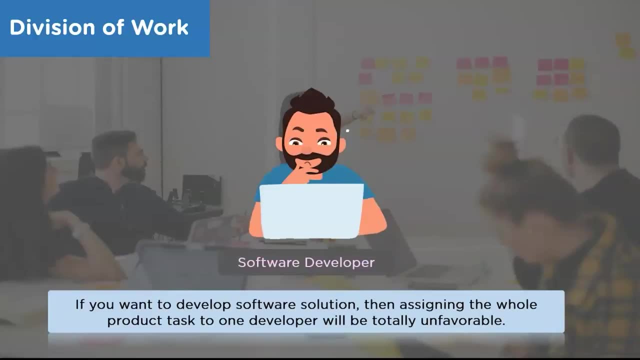 profession. As a result, the advantages of specialization will become available. Consider a software company that receives a project. They have also been urged to supply the entire project to a single software engineer for a period of time. It would now be extremely inefficient to assign the entire project to the single software engineer. Also, if 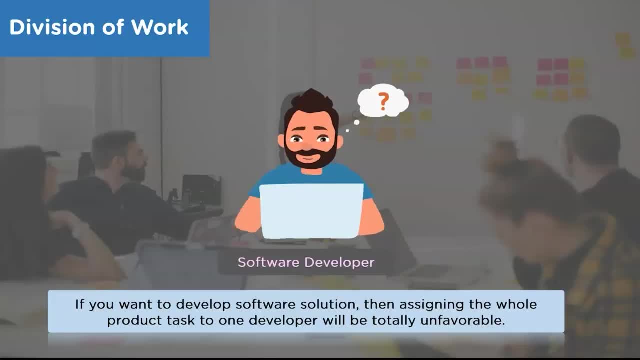 he encounters an error that he is unsure how to resolve, then it will be nearly impossible to finish a project before the deadline. Thus, rather than giving the whole project to the single specialist companies should assign it to the entire developer team By applying: 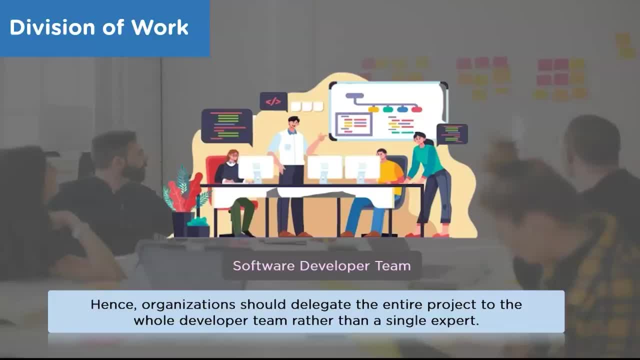 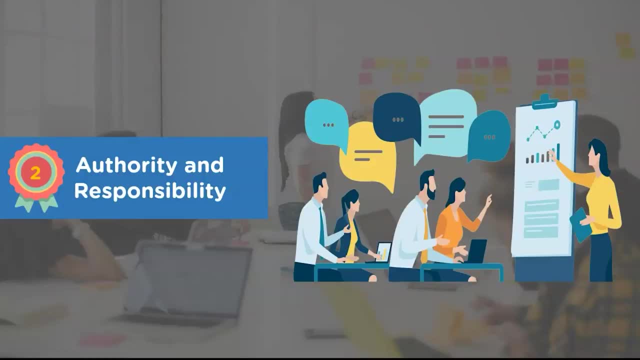 this division of work principle, the companies will be able to finish their project before the developer team. Next up is Authority and Responsibility. Fayol believes that the authority and accountability to issue instructions should be placed in the hands of few people and should not be. 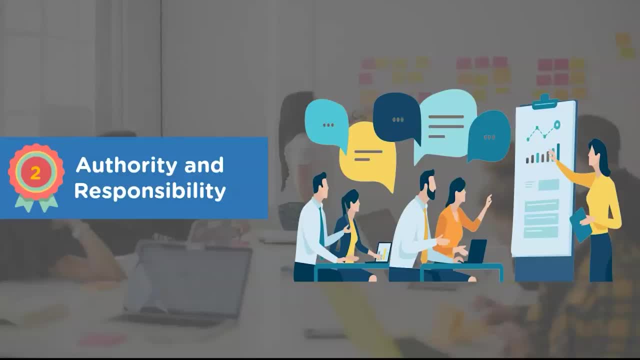 delegated. One of the most typical mistakes made by major corporations is that their management consists of too many people, thereby creating conflicts. When a few hand-picked persons have the power to vote, this authority gets transferred down the chain. With such authority comes a great deal of responsibility. Assume you are the marketing. 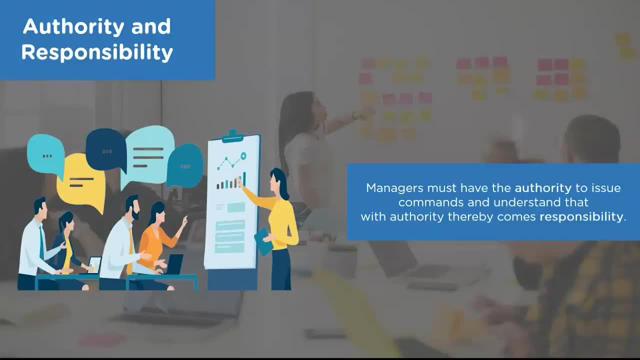 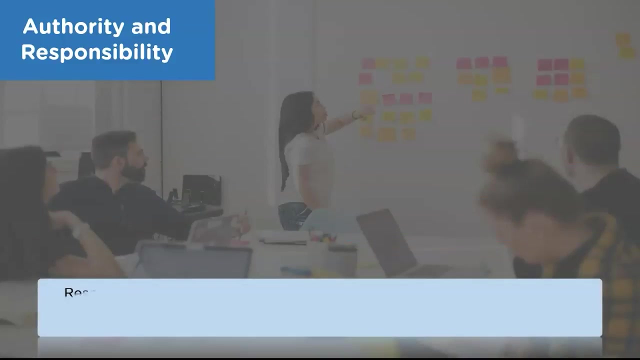 director of a corporation and you make a decision to sell a specific product. If the product fails, you must accept responsibility for the failure. You can't blame someone else As a result. when a person accepts responsibility, he also makes good decisions. That is why. 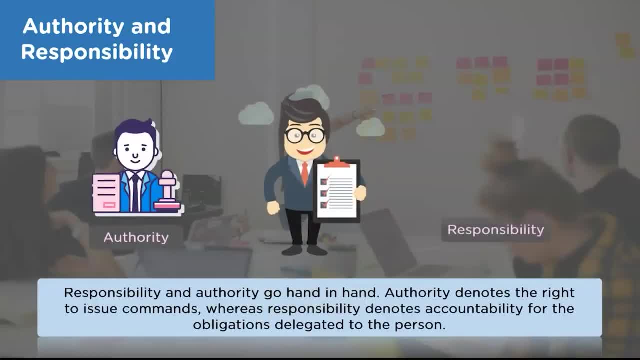 Fayol suggests authority and responsibility should go hand-in-hand. This is why, when a person accepts responsibility, he also makes good decisions. That is why Fayol suggests authority and responsibility should go hand-in-hand. This is why, when a person accepts responsibility, he also makes good decisions. That is why. 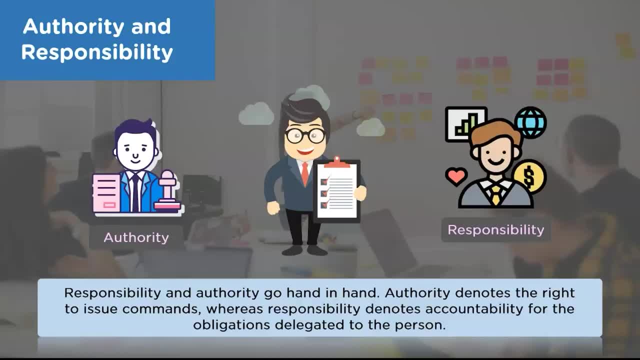 Fayol suggests authority and responsibility should go hand-in-hand. It means that when a particular individual is given a particular work, then he will be responsible for the results. This is only possible when he is given sufficient authority to discharge his responsibility. The right to give instructions is denoted by authority. 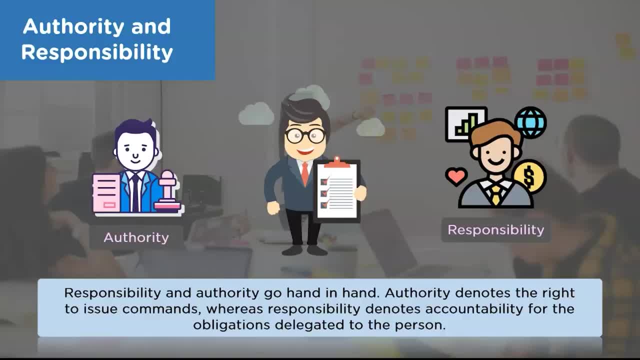 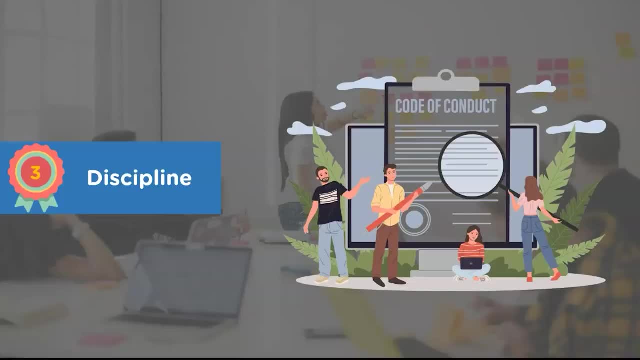 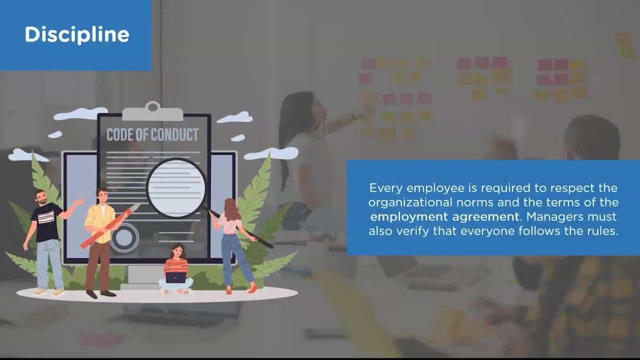 whereas responsibility denotes accountability for the obligations delegated to the person. The third principle on our list is Discipline. According to this principle, management should be accountable for how an organization's discipline is maintained, and this discipline percolates all the way to the bottom of the employee chain. Every employee must respect the organization's. 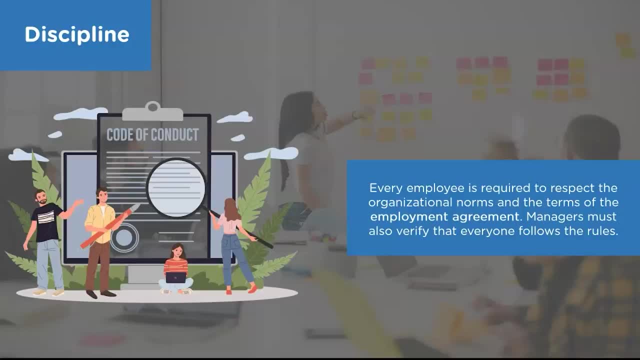 norms and terms of the employment agreement, and the validation of this should be done by a manager at each level. A manager can set a positive example for his staff by disciplining himself at first. Ad agencies are a good illustration of this. Ad agencies are a good illustration of this. 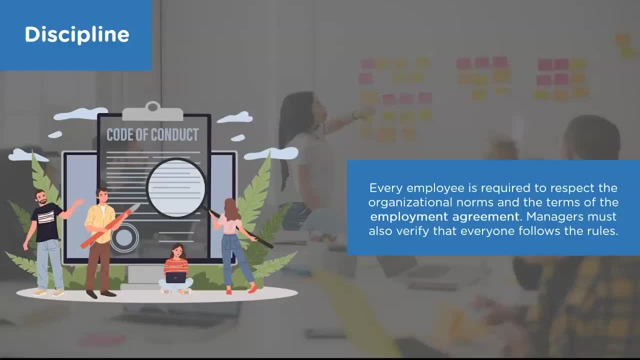 As they encourage informal meetings and chats in order to create better ties with their consumers. although these ad companies are known to retain discipline in the way ad executives engage with customers or carry out their business, Discipline is part of the organization's mission and ideas. Thus, it should be preserved and followed. 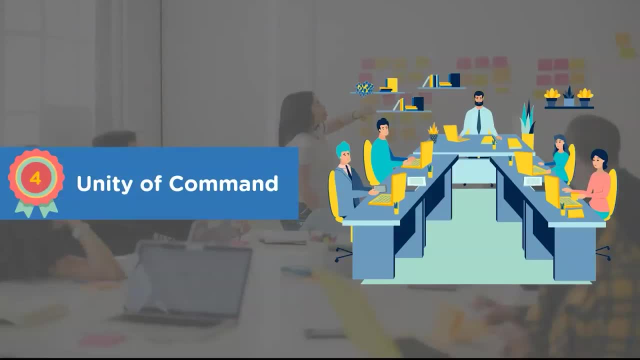 Next up is Unity of Command. When we examined authority in the previous principle, we stated that authority should be a part of the organization's mission and not a part of the organization's mission. The authority should be limited to a few people. Similarly, authority travels down the chain. 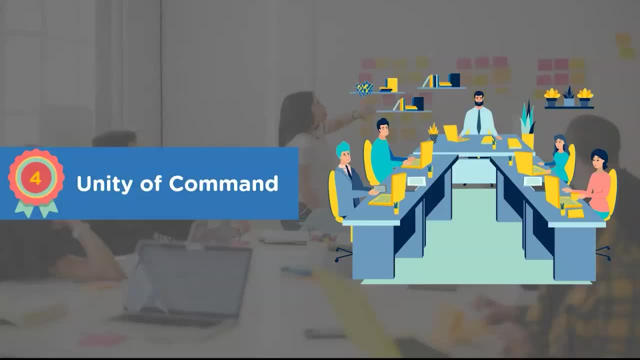 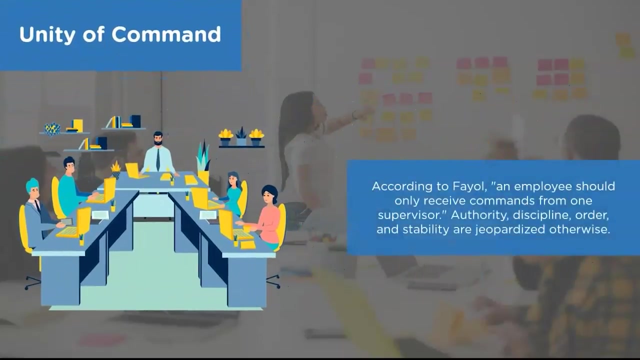 only when the authority individual is affiliated with a small number of people. If everyone in a political party reported directly to the prime minister, then he would be in hospital soon due to the high amount of stress As a result. there is a hierarchy in place to 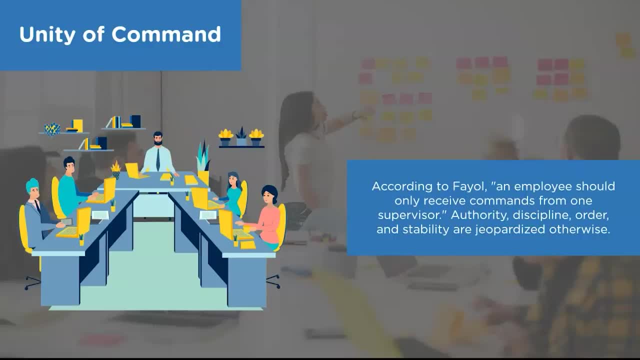 sustain a command. One person should only report to one leader, not two, three or four. Thus more and more leaders should be in charge of the organization. Thus more and more leaders should be in charge of the organization. Thus more and more leaders should be in charge of the organization. 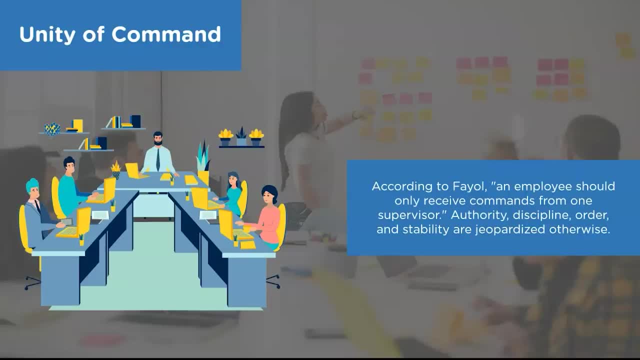 Most firms maintain the usual structure of national managers, regional managers, group managers and team leaders. This ensures that managers and executives know who they report to at all times, as well as their responsibilities and the performance expected from them. When you have achieved unity of command and a unified hierarchy where everyone knows. 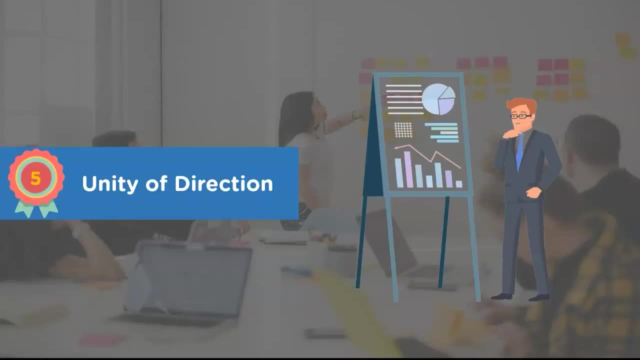 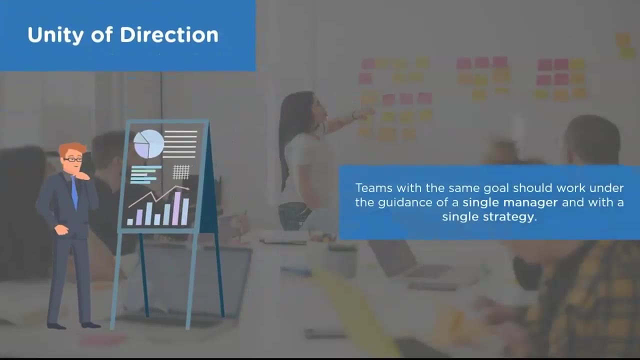 who they report to and is ready to perform the leader's bidding. it is time to adopt unity of direction. The term unity of direction refers to the presence of one person in charge of one plan to attain the organization's goal. In other words, there should be one plan of action. 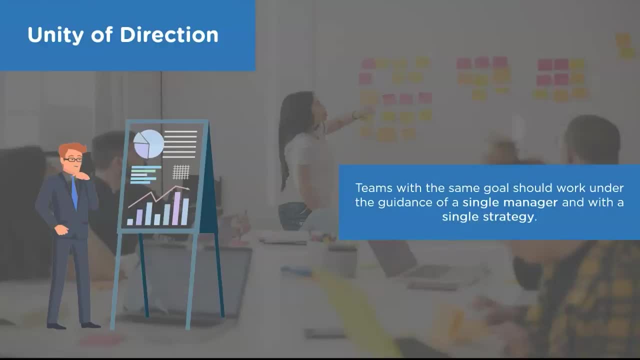 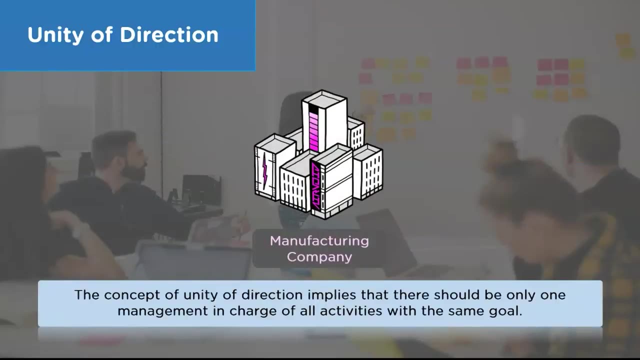 for a set of activities with the same goal and one manager to oversee them. For example, consider an automobile firm that manufactures two items, namely bikes and cars. Hence it has two divisions, Since each product has its own marketing strategy. each 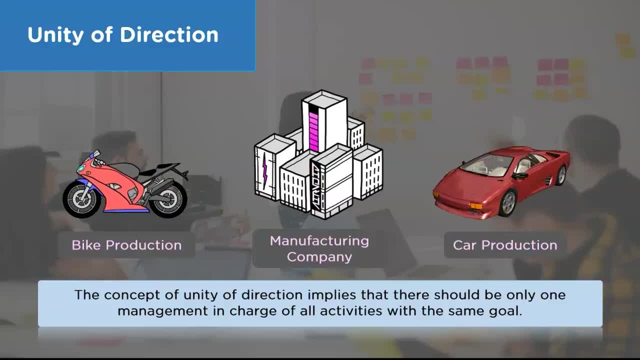 division must have its own set of goals To get positive benefits. each division must now plan its targets depending on its environment factors. It is vital to distinguish between the meanings of unity of command and unity of direction. The term unity of command refers to the fact that only one manager should be giving orders. 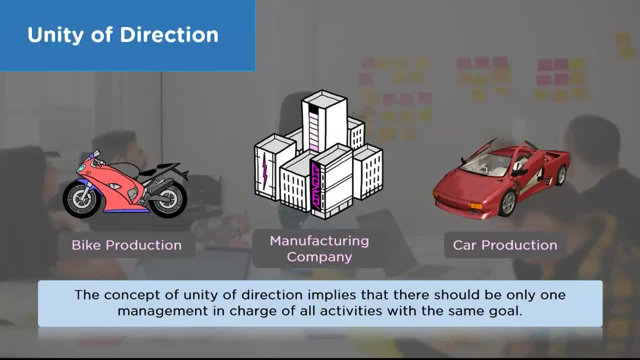 to an employee at any given time, And unity of direction refers to the fact that only one manager should be exerting control over all the operations with the same goal. The term unity of command refers to the fact that only one manager should be giving orders. 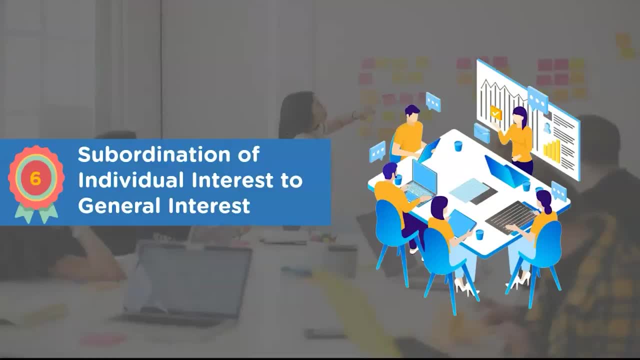 to an employee at any given time, And unity of direction refers to the fact that only one manager should be giving orders to an employee at any given time. Next on our list is the subordination of individual interest to general interest. This principle can also be named as priority to general interest over individual interest. According to this, 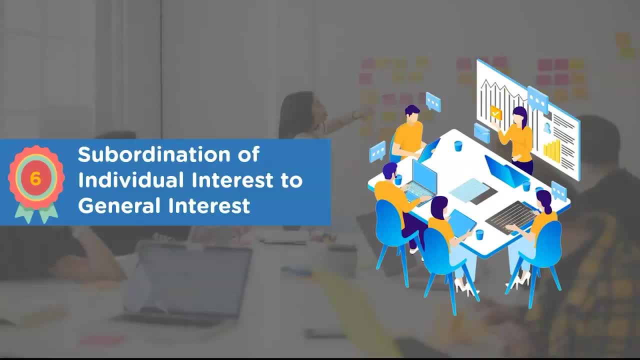 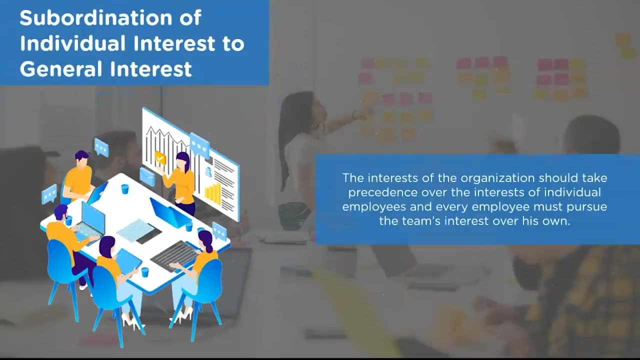 principle, the general interest or the interest of the organization should take precedence over anything else. Many times a person is fired from cooperation because he is moonlighting or performing to complete his own agenda. This is because the corporation wants to ensure that everyone who works for them is fully committed to the organization- The organization's- 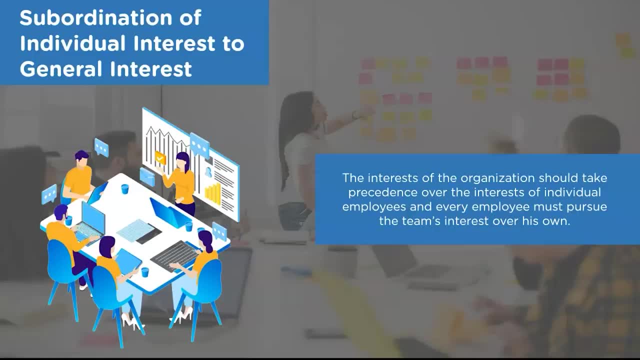 focus is on individuals, who give their all to the enterprise. That is why Fayol suggests that the company's interest should take precedence over the individual's. For example, suppose a manager makes a decision that hurts him personally but results in significant profit for the firm. In that case he should undoubtedly prioritise the company's interest. 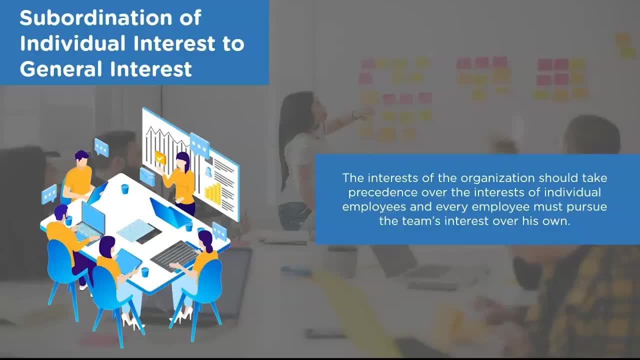 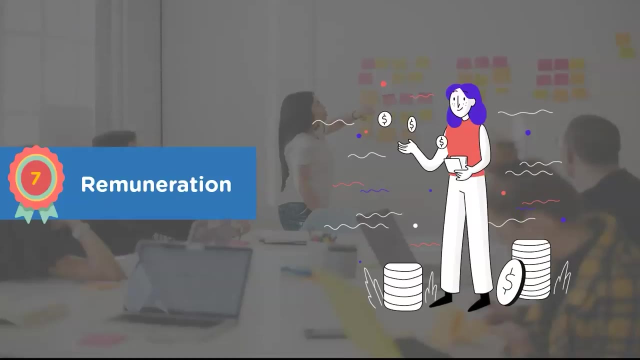 and make the decision appropriately. On the contrary, if a decision benefits the manager personally but results in significant loss for the company, then it should never be made. The seventh FAYOL principle of management is remuneration: When you expect your staff. 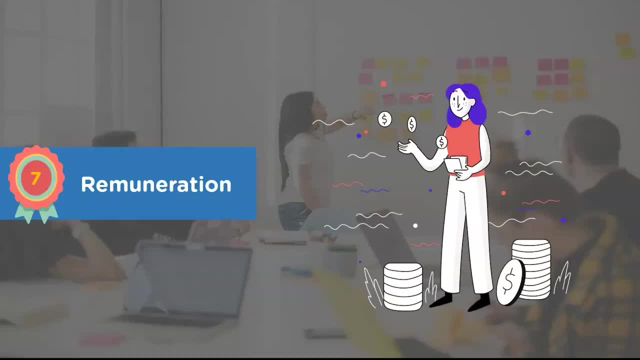 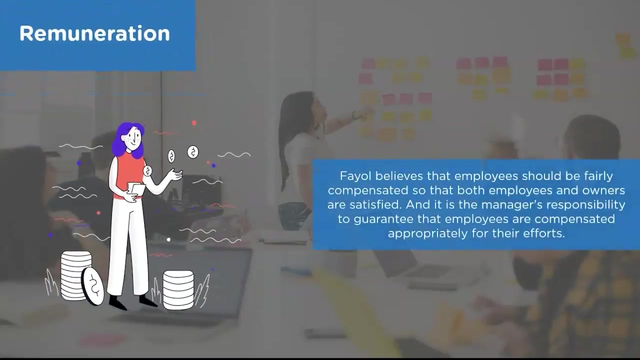 to be disciplined and want the unity of direction and command. you must compensate them so that they are less involved, inclined to shift to the competition and more likely to focus on the responsibilities at hand. Fayol believes that employees should be paid fairly to have the same level of pleasure. 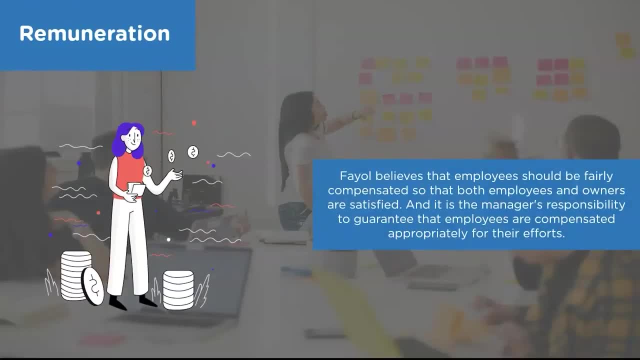 between employees and owners. The manager is responsible for ensuring that employees receive pay for their efforts, but if they are not appropriately rewarded for their work, they will not do their work with perfect dedication, integrity and capacity. Fayol believes that some monetary and non-monetary incentives should be provided to inspire employees. 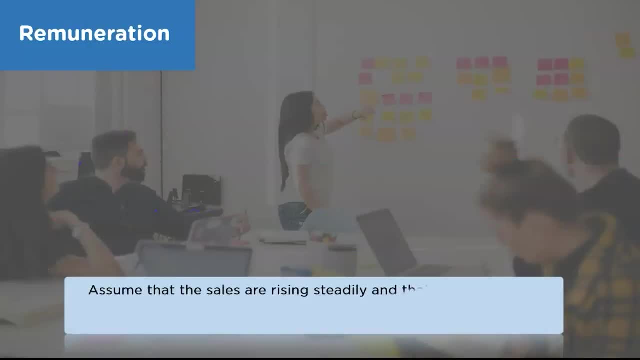 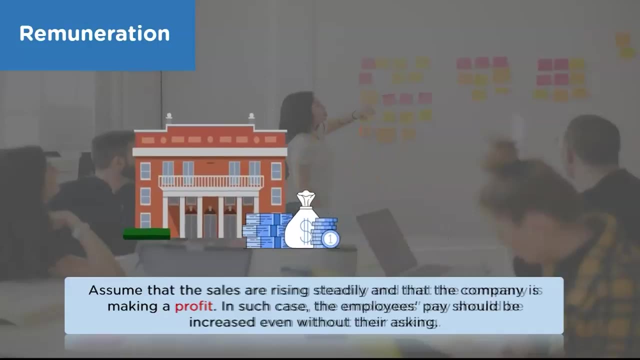 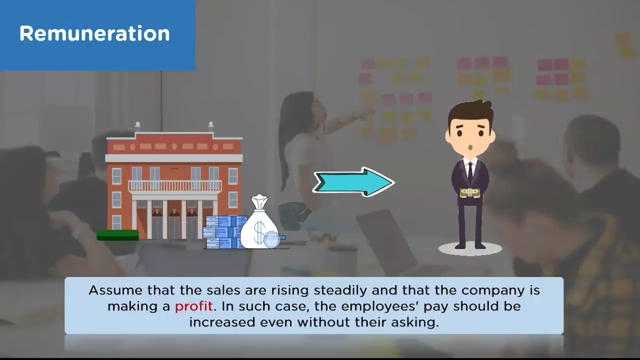 other than basic compensation. Assume, for example, the market is getting dearer and dearer to the organization and it is making high profits. In such case, the employees' pay should be increased, even if they do not request it. If this is not done, the staff will quit the firm as soon as possible and the expenses 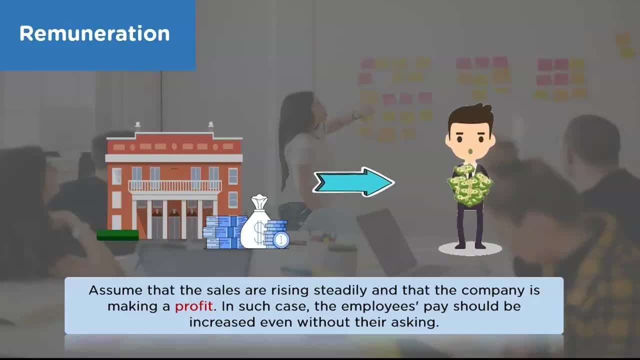 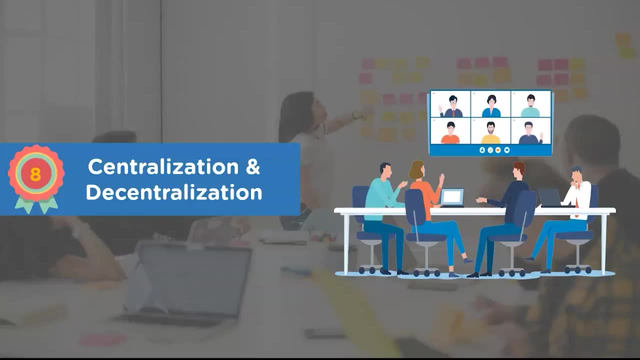 for new hires will be increased. This will result in a loss for the firm. The next principle of management is centralization and decentralization. According to this theory, superiors should use effective centralization rather than total centralization or total decentralization. 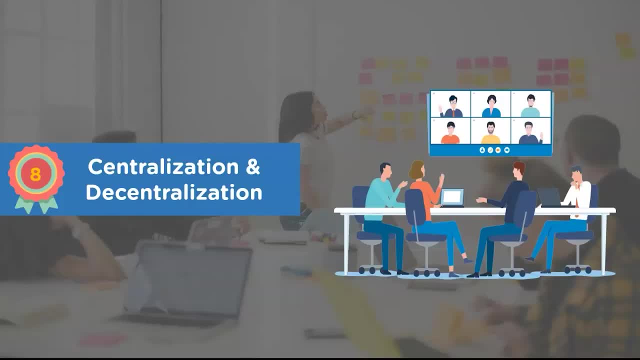 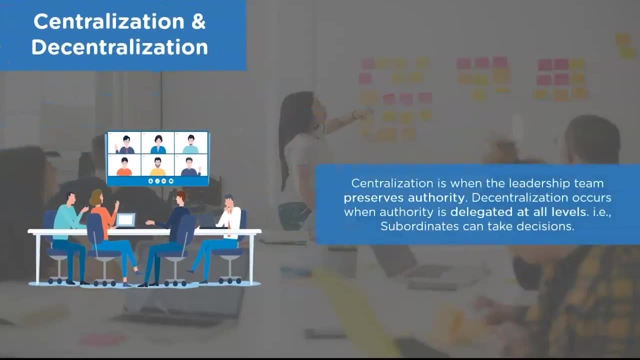 Fayol does not intend that authority should be entirely centralized when he says effective centralization. The degree of power that people in the organization have is referred to as centralization. The degree of power that people in the organization have is referred to as centralization. 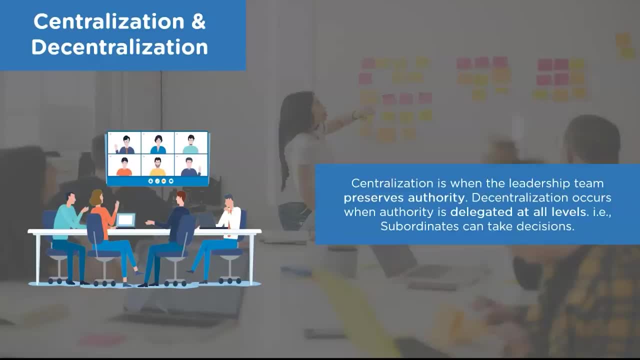 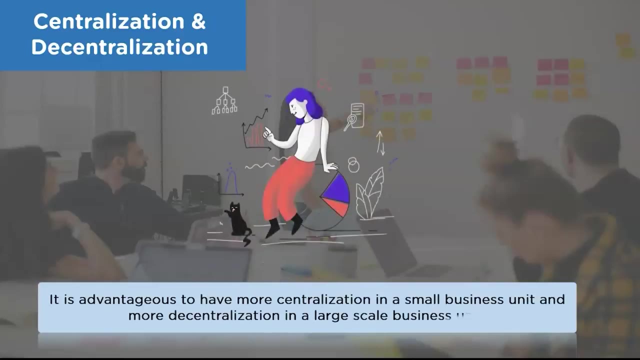 Centralization occurs when a small group of people exercise power over a larger group of people, And decentralization, on the other hand, occurs when a bigger percentage of people in the organization have a control, For example, decisions on objectives and policies, business expansion and so on, should remain. 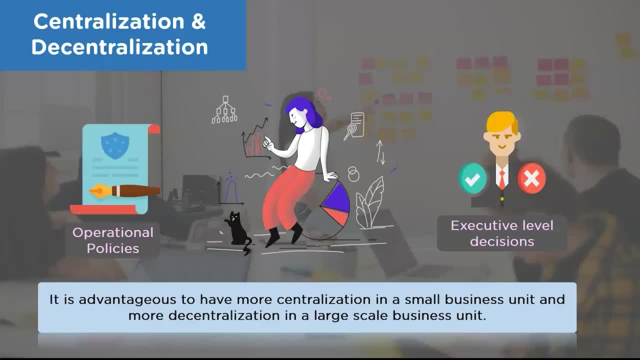 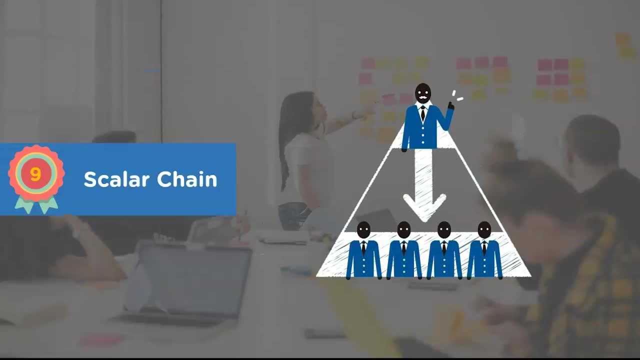 in the hands of superiors. On the other hand, authority for purchasing raw materials allowing staff leave should be entrusted to the superiors. The ninth principle of management is scalar chain. Many people are confused by scalar chain, But let me simplify it for you. 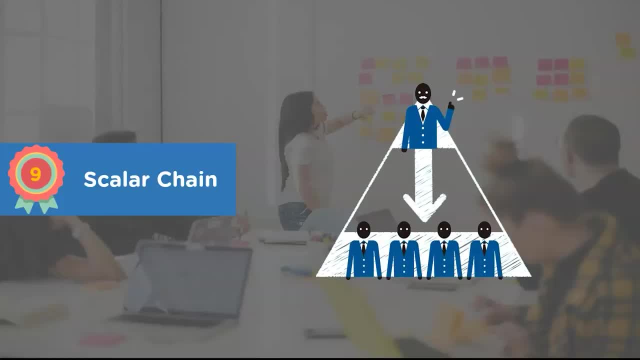 When discussing command and control, I stated that one employee should only report to a single manager higher up the chain. Hence an executive reports to a team manager, who reports to the regional manager, who reports to the national manager, and so on. 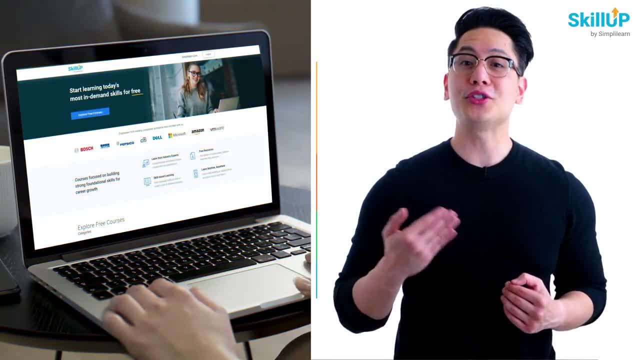 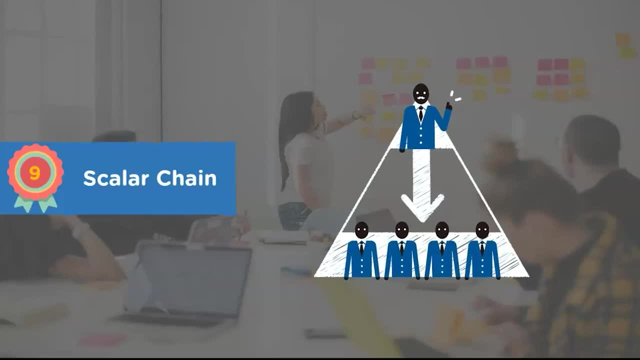 If getting your learning started is half the battle, then you need to know how to manage your team. And if you don't have the battle, what if you could do that for free? Visit ScaleUp by SimplyLearn. Click on the link in the description to know more. 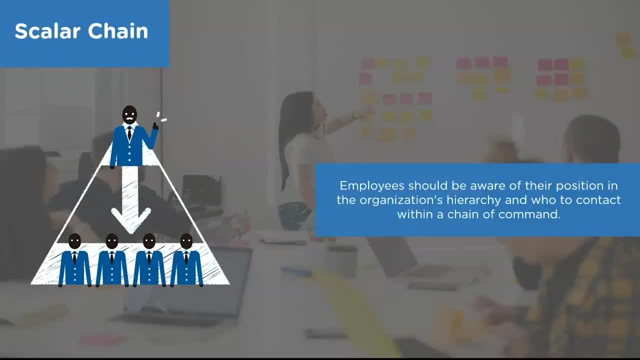 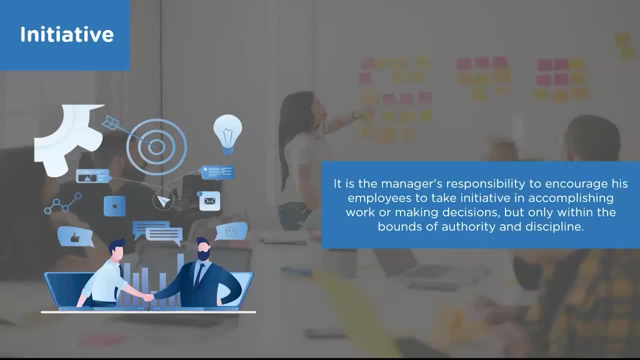 his workers when it comes to completing work or making decisions, but only within the bounds of authority and discipline. It will be only conceivable if the manager welcomes the ideas of his or her colleagues. Support Nets will continuously propose their fresh and beneficial ideas as a result, and 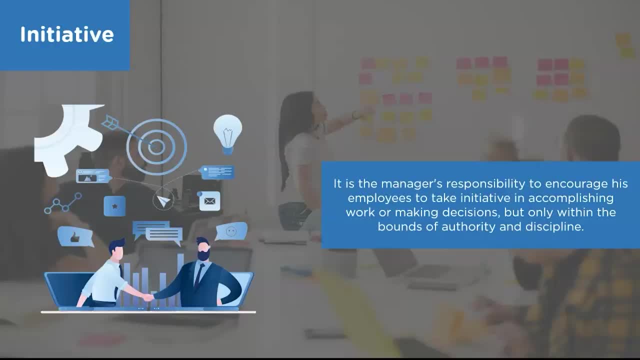 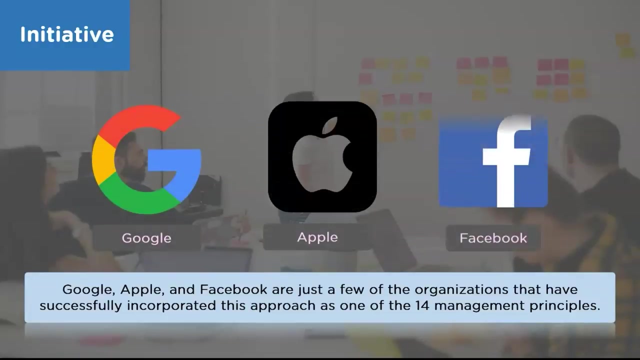 they will eventually become an essential part of an organization. To make this procedure a success, a manager must let go of his false feeling or grandeur. Google, Apple and Facebook are just a few of the firms that have successfully applied this concept amongst the 14 management principles. 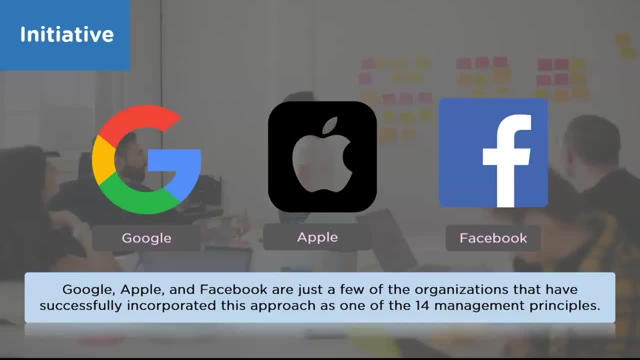 Developers and engineers at Google are allowed their own sweet time to find out creative approaches that can be implemented as products in Google. The same is true for Facebook and Apple. Because employees are encouraged to take the initiative, these businesses have a high degree of creativity. 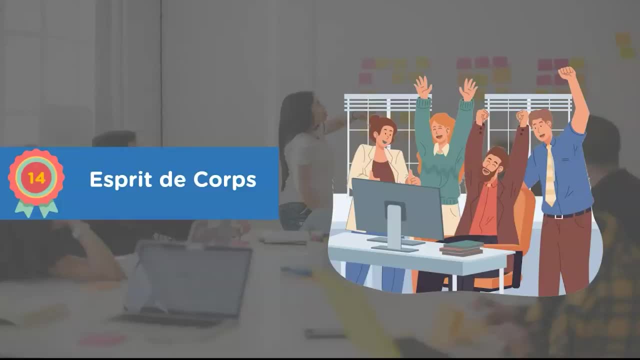 The last Henry Foyle principle is ESPIRIT DE CORPSE. The term ESPIRIT DE CORPSE refers to a sense of pride and mutual devotion felt by members of a group, and it is just what you must strive towards if you want to attain success, while 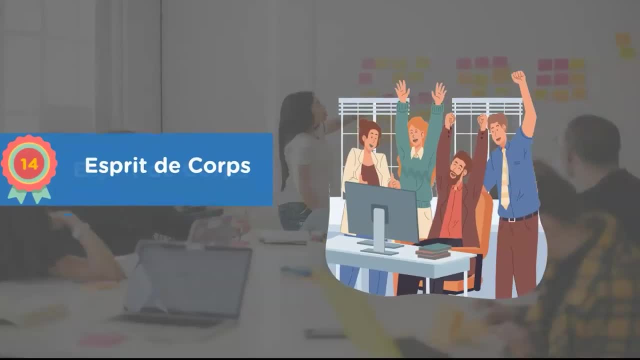 employing the 14 principles of management. ESPIRIT DE CORPSE. ESPIRIT DE CORPSE IS THE ULTIMATE UNION OF MANAGEMENT. ESPIRIT DE CORPSE IS THE ULTIMATE UNION OF MANAGEMENT. ESPIRIT DE CORPSE IS THE ULTIMATE UNION OF MANAGEMENT AND EMPLOYEES INSIDE AN ORGANIZATION. 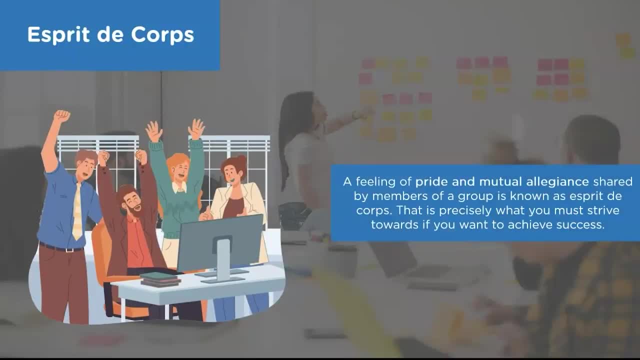 RESULTING IN A COMPANY THAT IS PROUD OF WHAT IT DOES AND HAS A LOT OF LOYALTY FROM ITS EMPLOYEES AND CUSTOMERS. ONLY A FEW FIRMS HAVE BEEN ABLE TO DO THIS. FEW OF THEM ARE INTEL, APPLE, AMAZON AND SAMSUNG. 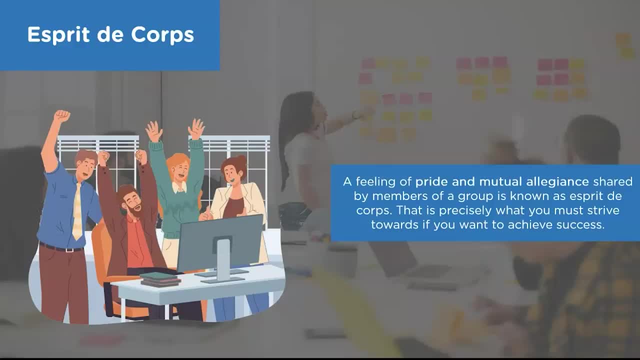 IF A FIRM BECOMES ABLE TO IMPLEMENT ESPIRIT DE CORPSE, THEN IT PROVIDES IT A LEGITIMATE COMPETITIVE AGE, SINCE IT INDICATES THAT THE EMPLOYEES ARE PASSIONATE DRIVEN AND 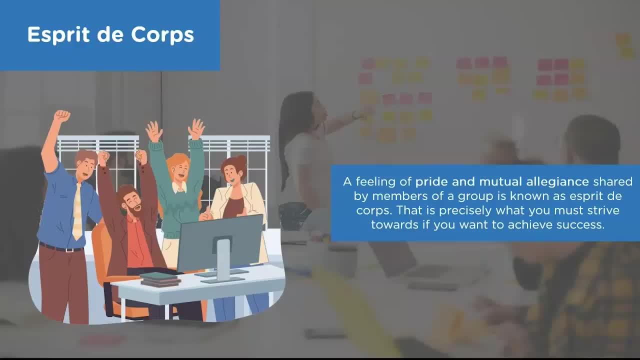 WILLING TO GO ABOVE OR BEYOND FOR THE FIRM OR MANAGEMENT OVERALL. THESE 14 MANAGEMENT PRINCIPLES ARE EVERGREEN IN NATURE, NO MATTER HOW QUICKLY TECHNOLOGY CATCHES UP WITH US. THESE 14 MANAGEMENT PRINCIPLES WILL. 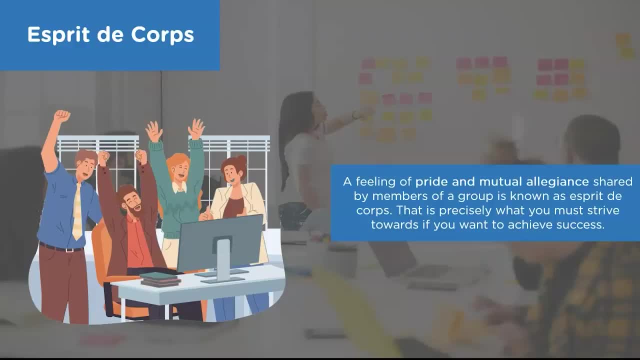 MATTER TO EVEN THE SMALLEST OF BUSINESSES AND HELP THEM BECOME ENORMOUS. THERE ARE EVEN EASIER WAYS TO KEEP TRACK OF SOME OF THE SUBJECTS INCLUDED IN THE 14 MANAGEMENT PRINCIPLES. HOWEVER, THE ULTIMATE AIM IS TO CREATE A COMPANY THAT IS ABLE TO IMPLEMENT ESPIRIT DE CORPSE. 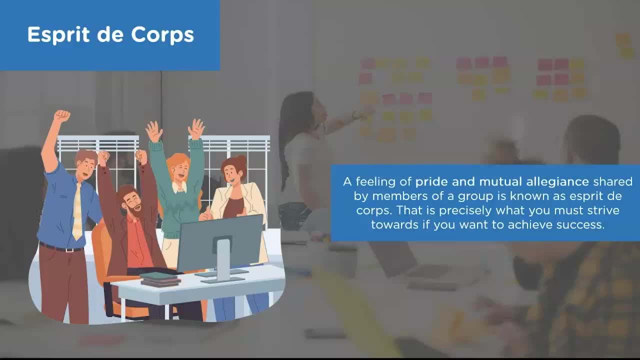 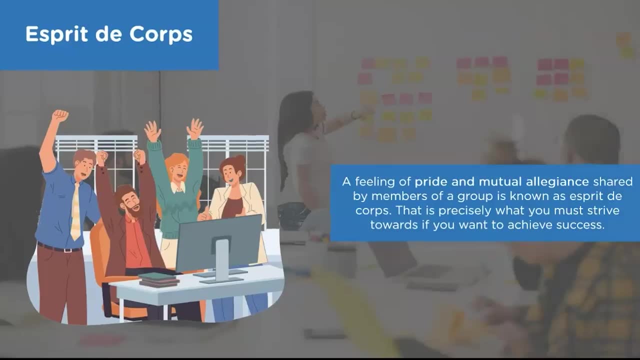 AND CREATE AN ORGANIZATION THAT IS EFFICIENTLY MANAGED, PRODUCTIVE AND DELIVERS THE BEST OUTCOMES POSSIBLE, IN ACCORDANCE WITH THE COMPANY'S GOALS. I HOPE THESE BASIC PRINCIPLES OF MANAGEMENT ARE CLEAR TO ALL OF YOU OUT THERE. 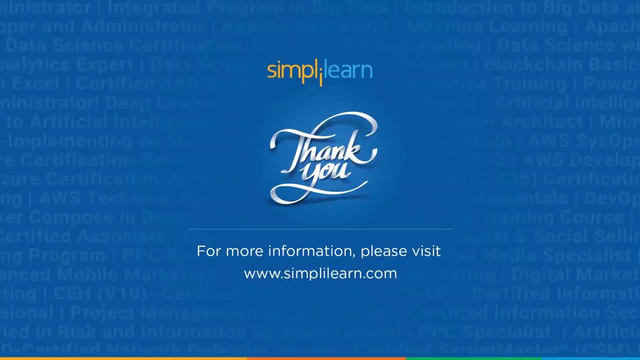 THAT'S ALL WE HAVE FOR TODAY. IF YOU HAVE ANY QUERIES REGARDING THE TOPICS COVERED IN THIS SESSION, THEN LET US KNOW ABOUT THEM IN COMMENT SECTION BELOW, AND OUR TEAM OF EXPERTS WILL GET BACK TO YOU. THANK YOU SO MUCH FOR BEING HERE AND DO WATCH OUT FOR MORE VIDEOS.